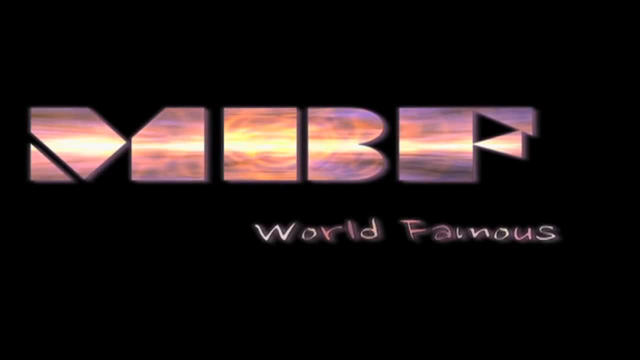 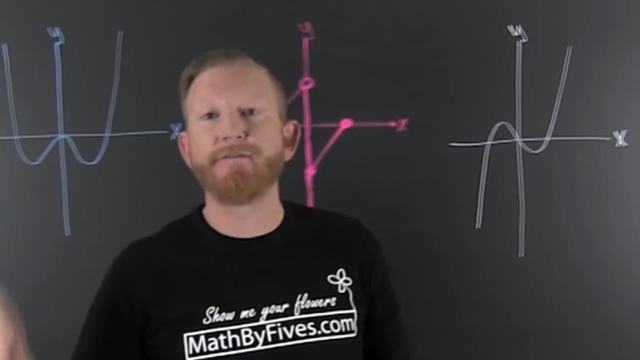 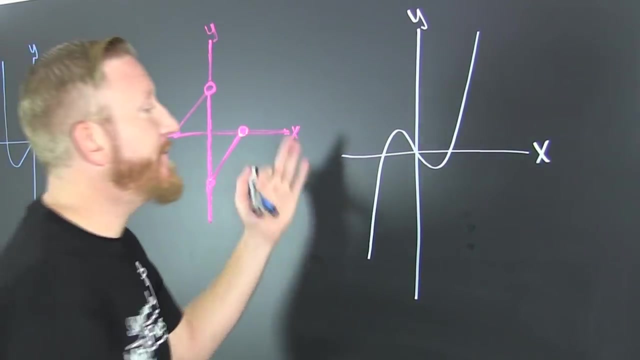 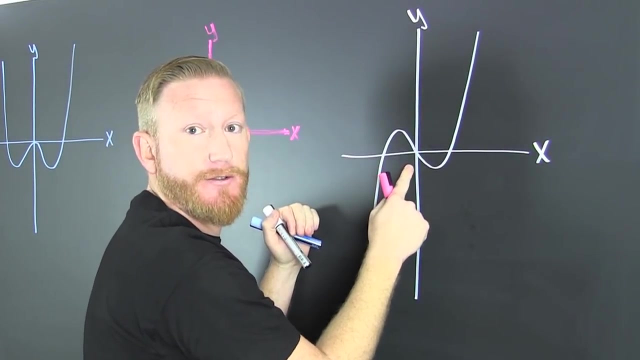 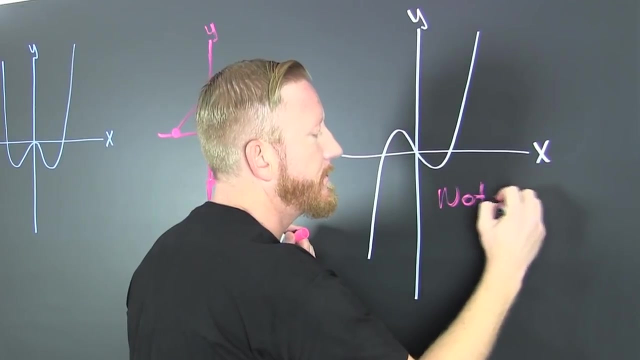 Even odd or neither From a graph. Ah, Let's go back over here, Bam. Okay. So a function is, even if it has x-axis or y-axis symmetry. Does this have y-axis symmetry? Is it same on the left as it is on the right? No, So this is not. even Come on pink. Oh the struggle. 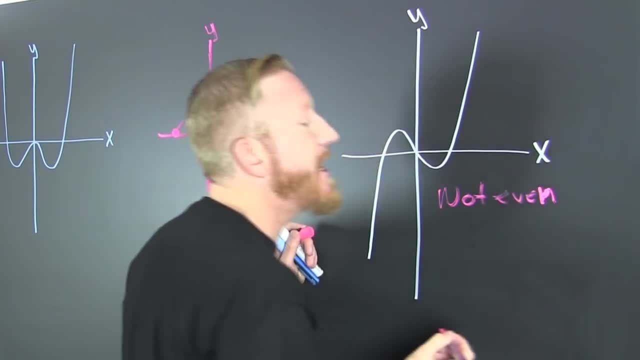 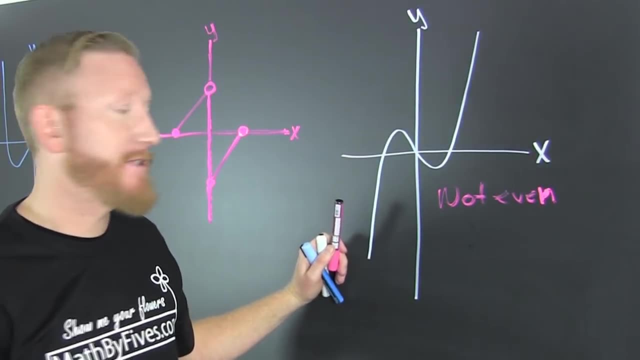 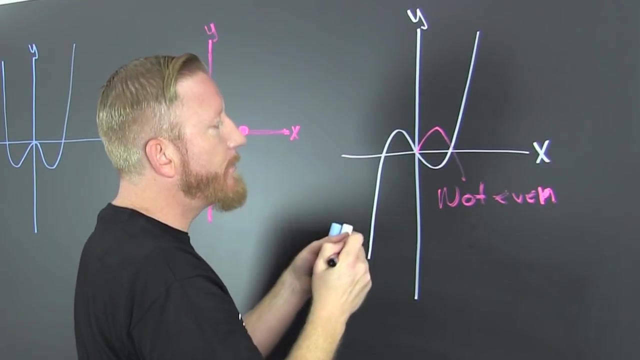 is real. That's not even. Did I fix it, I don't know. So now we check to see odd. It's odd if it has origin symmetry. So we flip it across the y Bam, And then what Then? 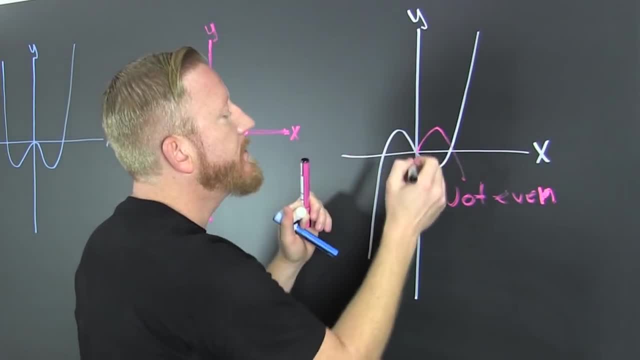 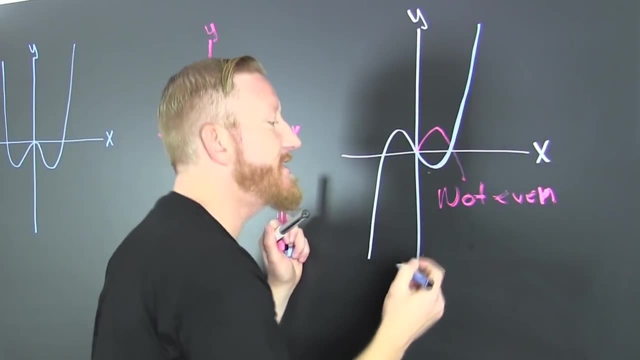 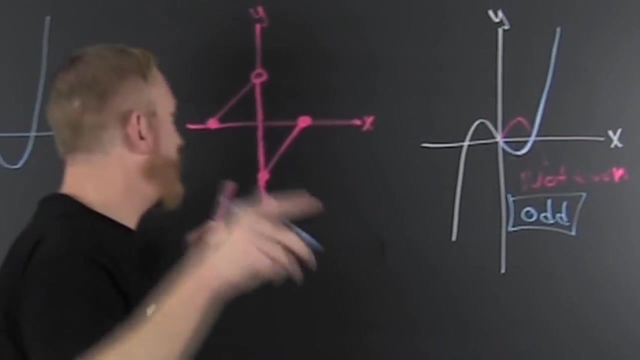 we flip it across the x, Then we flip it across the x. So does it lie on itself? Sure it does. So this is odd, You're odd. Okay, Bam, This one Whoa. So we check to see. 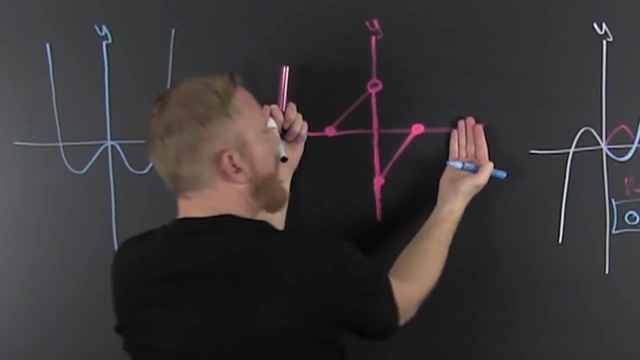 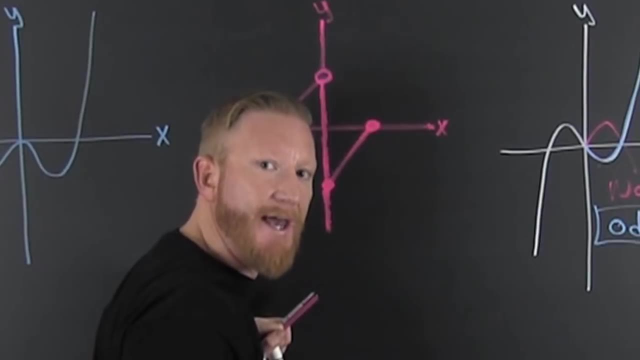 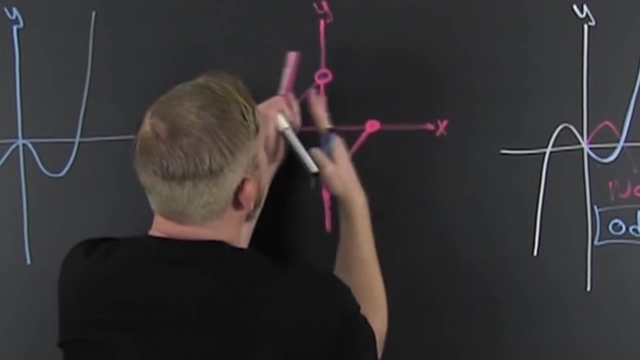 if it has x-axis symmetry, Alright, why? Because we're- I'm just messing this up- We're checking to see if it has y-axis symmetry symmetry. If it has y-axis symmetry, then it's. even If I fold it across the y, no, no, not the. 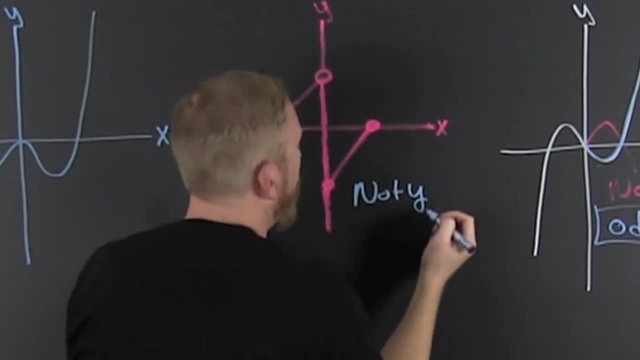 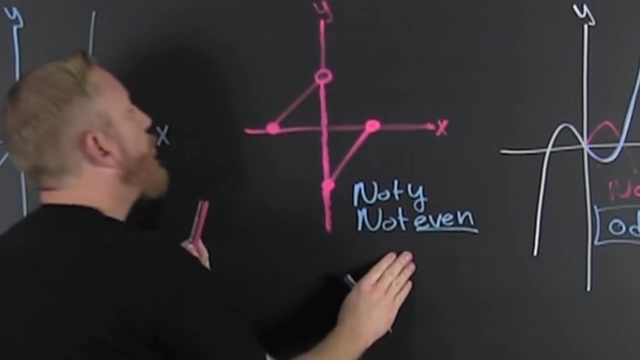 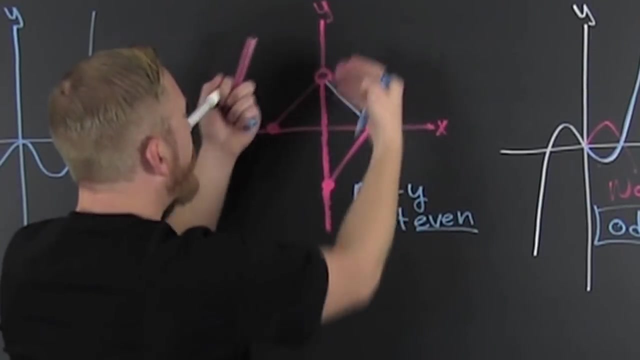 same, Not y, Which means not even Okay. so now I'm checking to see if it's odd. So we fold it across the y Bam, And then we fold it across the x Bam. Does it lie on itself? Yeah, except.